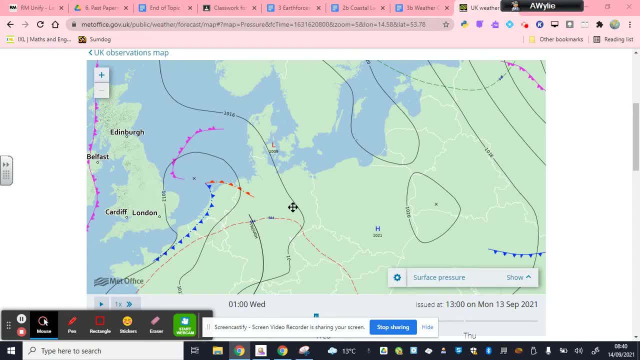 What does that mean? Well, once we know we're in high pressure, we should be able to figure out that the winds travel in a clockwise direction. So in Berlin, the winds are traveling along this ISA bar down here, and therefore, if I was sitting in Berlin, I would notice the winds coming from. 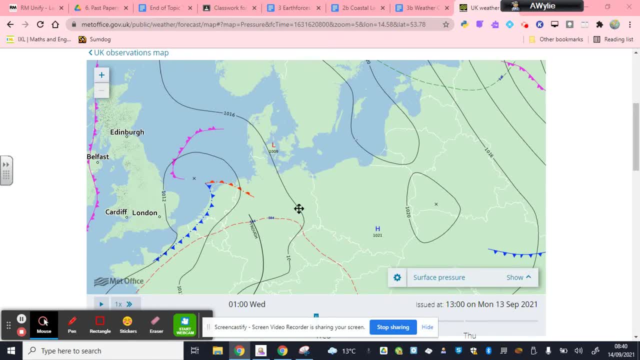 the northwest, because up here is the northwest and they're traveling down this way. So that's one aspect of the weather I'd be thinking about. Would the winds be strong? Not particularly. How do I know this Because the ISA bars are far apart. Is it raining? Well, it's highish. 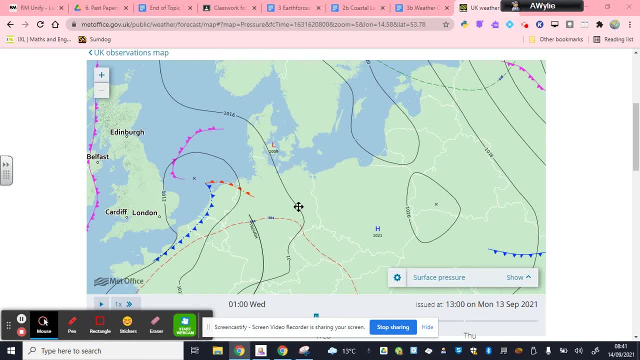 pressure, so there's unlikely to be many clouds in the sky and there are no weather fronts over Berlin. We can see some over here, over the Netherlands, but it's unlikely to be raining Now. what we can, however, see if we're looking at this weather map and we're sitting in Berlin. 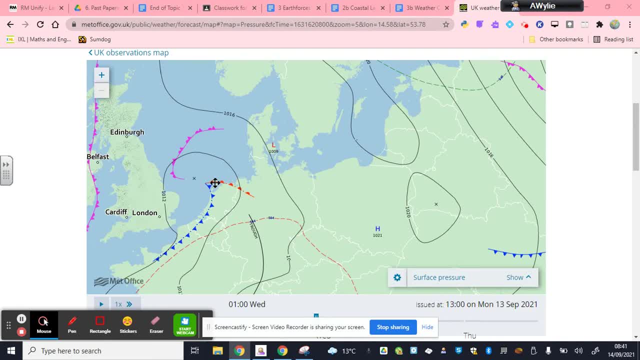 is over to our west is a warm front currently sitting over the western part of Germany and the northern part of the Netherlands, which is over here, and behind that is a cold front, And we do note a couple of things. We know about the type of rain that comes with warm fronts and cold fronts. 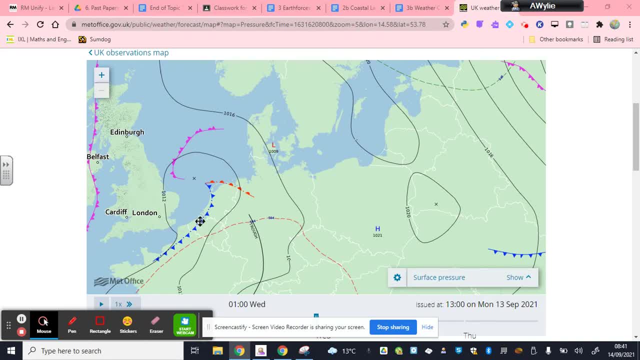 and we also know that these things generally- but not always, but generally- travel from west over here to east. So these two weather fronts have been probably on Tuesday, the day before, sitting somewhere over southern England, and they've now moved westwards and they're sitting. 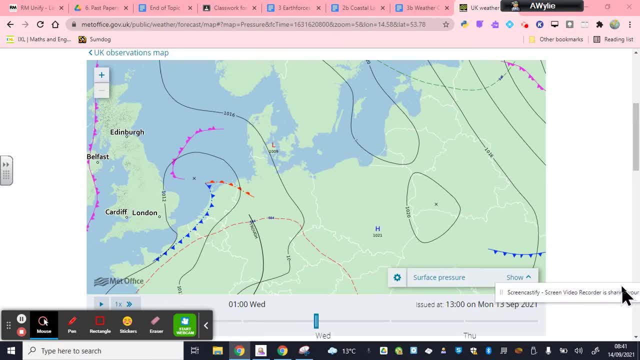 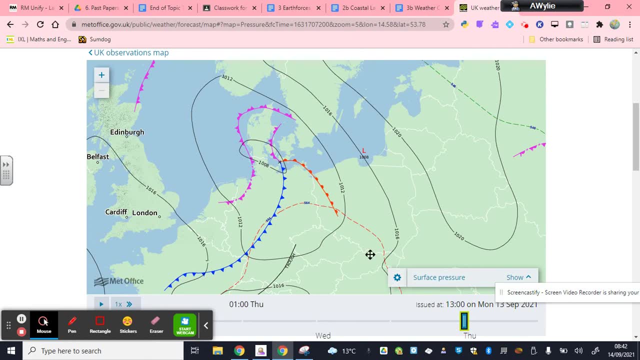 over the Netherlands. Well, let's just jump forward 24 hours to see what those weather- two weather fronts- have done. So we're going to go to Thursday and our map has changed. Okay, we are still in this area of reasonably high pressure. So, in terms of the wind direction, 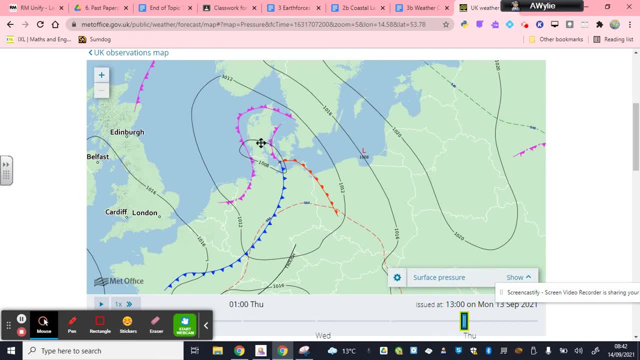 and the wind speed, we wouldn't be changing. particularly, Winds are still coming from the north in Berlin, or northwest, and they're not particularly strong. What has, however, changed is we can see that this warm front, which was over here a day before, has now moved hundreds. 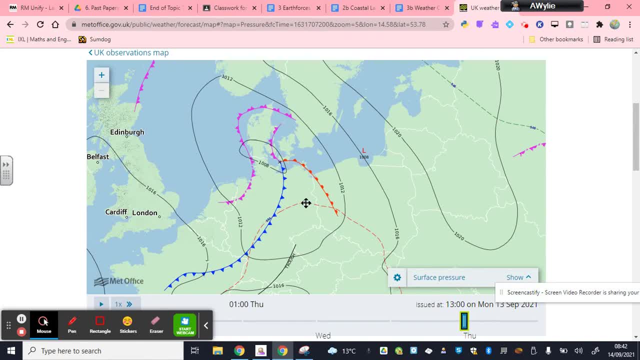 of miles across Germany and has actually passed Berlin now. So what we would know by a warm front on a Thursday at one o'clock in the morning, you see that there is, that Berlin has experienced steady rain, because we know that how Well, because a warm front is now sitting. 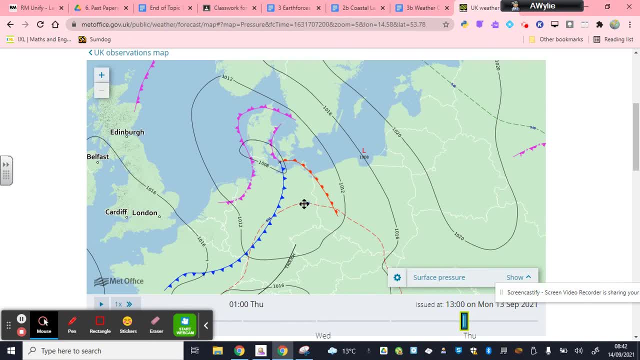 to the east of where Berlin is. The crosshair shows you where Berlin is and if it's lying now to the east but it was over here, it must have traveled across Berlin and warm fronts being steady rain. Another thing that will have changed is that the air temperature will have. 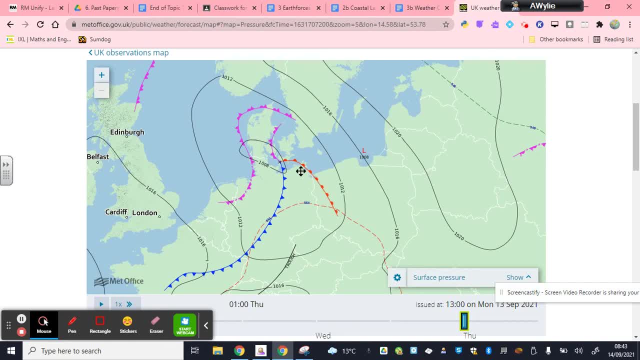 increased, because when a warm front passes overhead- and this rain passed overhead- it actually brought behind it- that's in this area- warmer temperatures. So Berlin is currently sitting in a warm sector and the warm sector is this area between- I'm just highlighting. 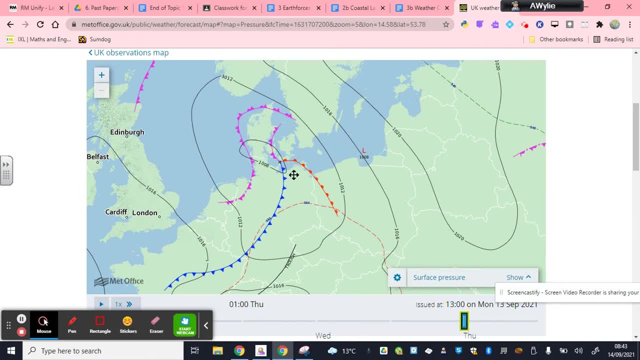 it with the cursor between behind the warm front and in front of the cold front. So the temperature has increased in Berlin slightly because the warm front has passed, but it has been steadily raining and it's likely if I was standing in Berlin when this weather map is showing. 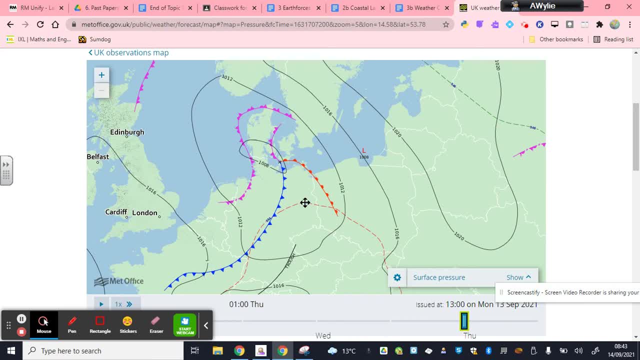 that I will have experienced rain a few hours before As the warm front passed. I might still be getting scattered showers, because that's what tends to happen between the warm front and the cold front, and I will largely. most of the sky will be covered. 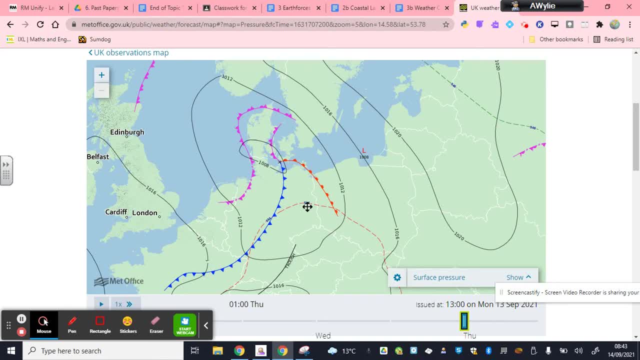 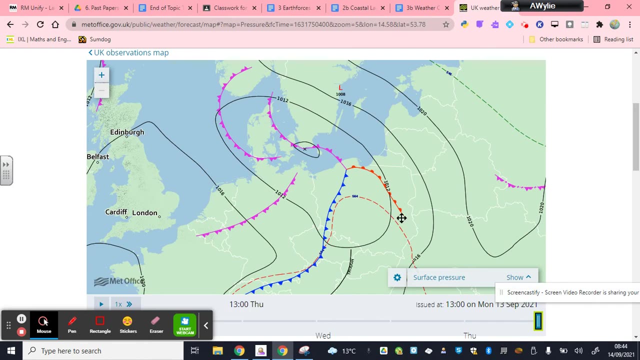 in cloud, with occasional breaks of blue sky, but it's going to be lots of scattered clouds with scattered showers. Now, what is going to happen over the next few hours, or 10 to 12 hours? Well, let's just go forward in time. What we can now see is that the warm and cold front which a day and a 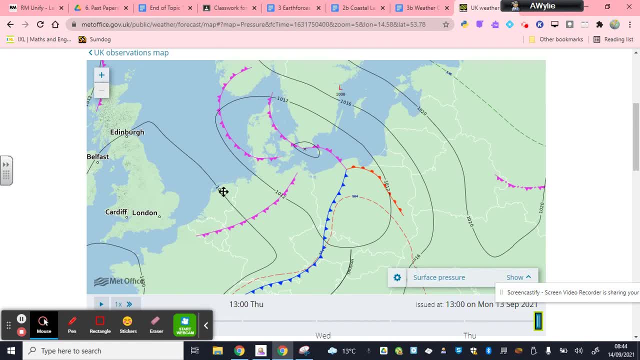 half ago were over here in Northern Holland, have now travelled over Berlin, which sits here, and now sit over Poland. There they are. they've changed shape slightly, but they're still the same thing. I can also see that the wind direction is starting to change slightly. it's now definitely. 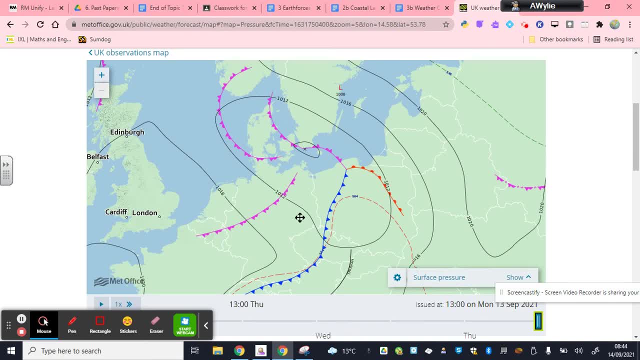 northwesterly. Actually, if you think, the wind's travelled clockwise, actually they're coming from the southeast to Berlin right now. So there's been a complete change of weather direction. the wind speeds are still pretty low because the ice is still quite high, but it's still pretty low. 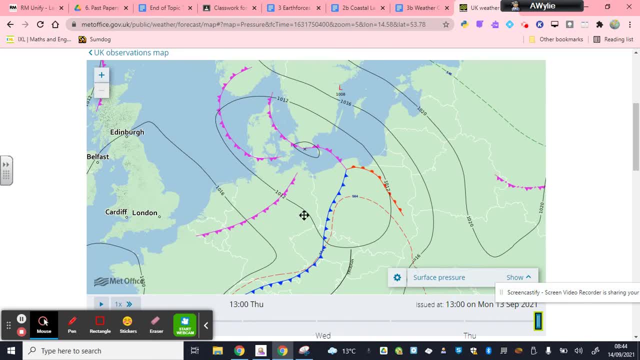 as far, as far apart. But what has been the big change? Well, this cold front here did pass over at some point over the night. We're at one o'clock on Thursday- well sorry, I should say mid-morning- and it will have brought a heavy downpour of rain in Berlin. That's the first thing that will have. 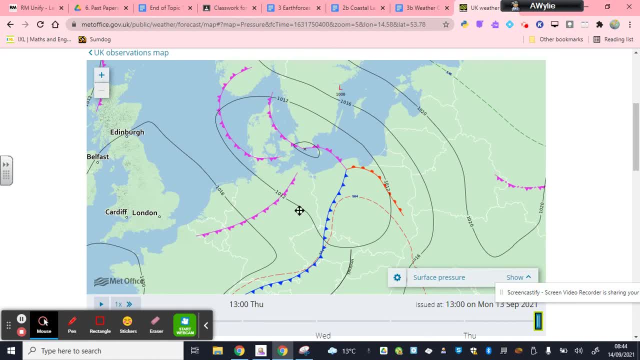 changed, So we've just experienced heavy rain. it's probably starting to clear up, although we now have another front coming in Now. this is a front that won't be talked about in National 5, it's called an occluded front and it brings very heavy rain, but you won't ever see that in a National 5 exam. Now, this is a front that won't be talked about in National 5, it's called an occluded front and it brings very heavy rain, but you won't ever see that in a National 5 exam. 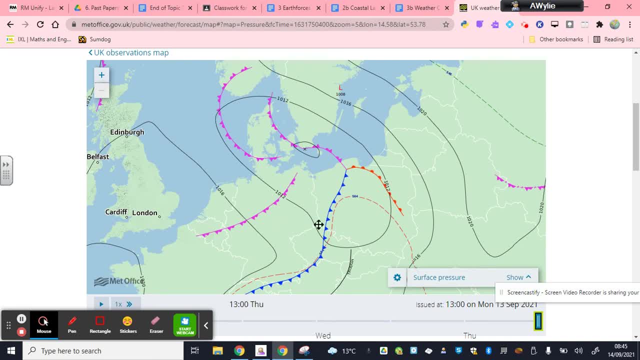 Now, this is a front that won't be talked about in National 5 exam, So let's just not concentrate on what's coming to Berlin, let's concentrate on the cold front. So we've had heavy rain in the last few hours and the temperature will have dropped because, unlike the air between the 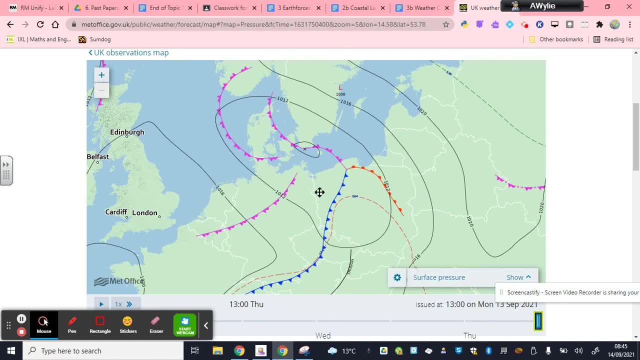 two fronts, which is warm in this, what we call warm sector. behind this front, and actually in front of the warm front, is always cold air. So this entire area that I'm tracking across is cold air, And this is actually an entire cold air mass that I'm just highlighting. 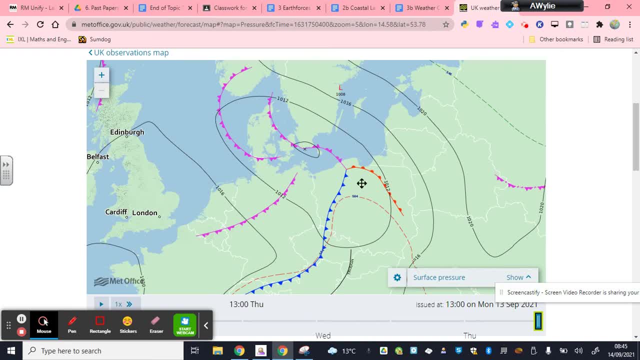 across the whole of this bit of northern Europe, Whereas on the other side of the warm front and this side of the cold front and this side of the warm front is warm air. So this is a warm air mass And you will remember that weather fronts are actually just the meeting point of 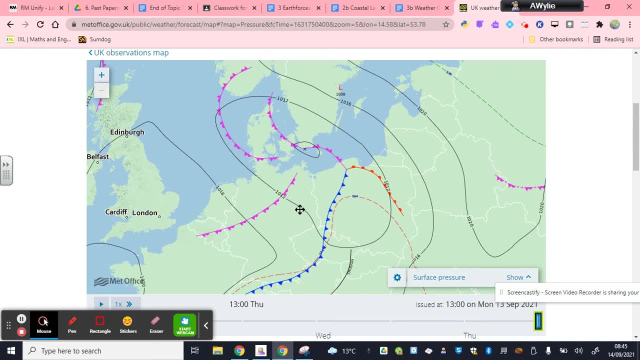 two air masses. So Berlin's temperature has dropped a lot. it stopped raining, probably, and it might have even cleared up temporarily. Wind directions changed completely, and that's just because the isobars are now in a different position, So the wind is still going clockwise. 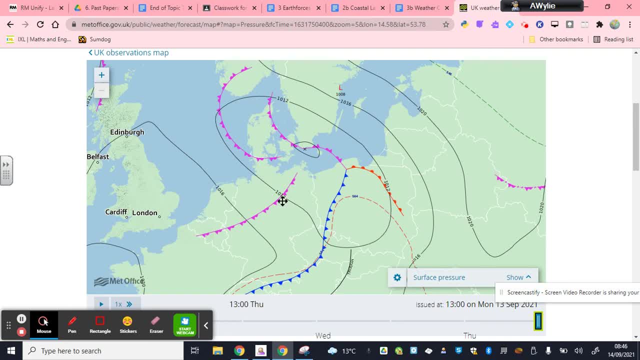 because it's high pressure, but it's coming from the south east now and traveling up this way. So what I have done in this tutorial is show you quite a complicated question that sometimes appears in exams: what happens or is likely to happen in the future. So if I was over here in 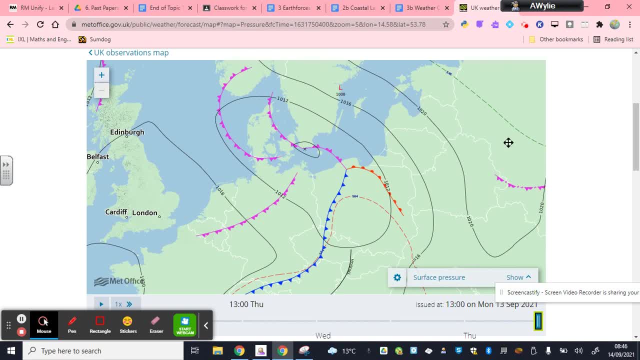 Moscow and you were asked what's the likely weather changes in Moscow, showing you where Moscow is? well, all you've got to do is look west on your map to see what's coming and then move all of this directly across to where you're going to be in 12 hours time, and that should help you. 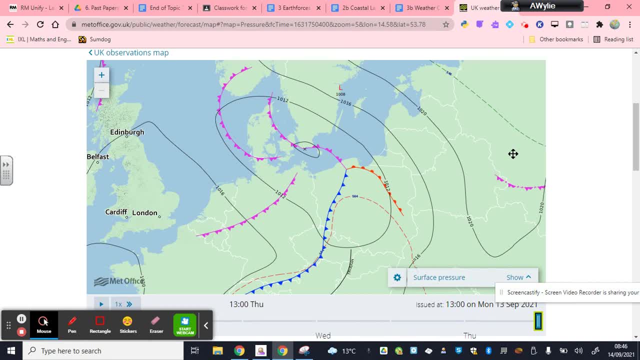 figure out wind direction changes and weather changes in terms of rain and temperature. So, of course, now I'm going to stop the video and show you about the weather. So what I have done is I have taken the weather forecast on my map. And it's coming back to normal only somewhere in 30 minutes. So now I'm going to come back to the forecast and I'm going to make a clear forecast. So the weather forecast on this map is: I used the weather forecast to show you the weather. forecast on the map, And what I'm going to do is I'm going to give you an idea of what's going on and I'm just going to quickly show you the weather forecast. So what's going to happen next?